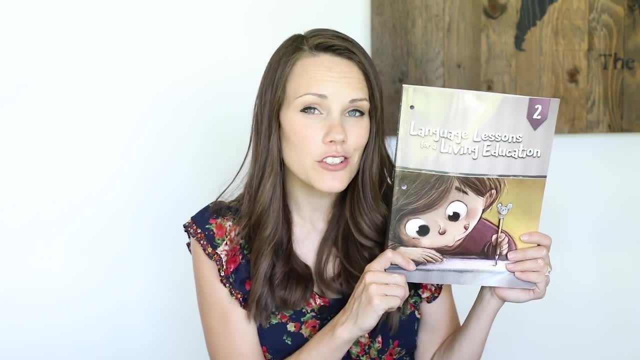 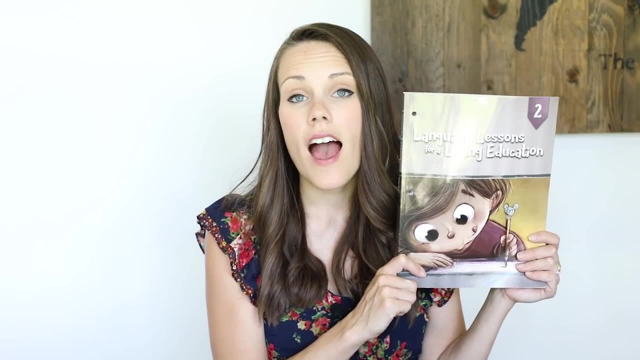 we know and love about Charlotte Mason, like picture studies and narration and dictation, But what really makes this unique is the fact that it's a curriculum that's not just about writing. It's a curriculum that is more of a lesson-based curriculum and that's 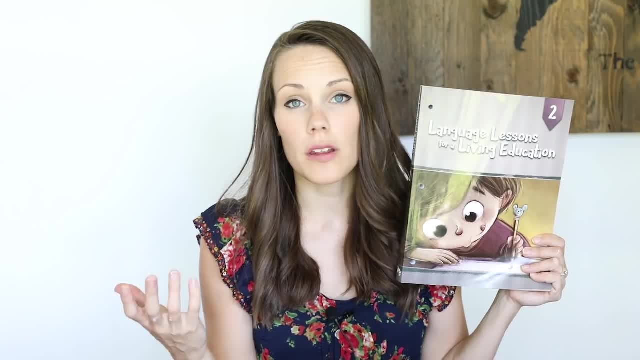 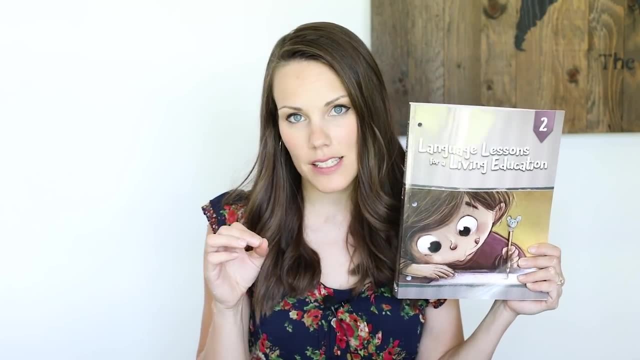 the way it's going to be, And the biggest thing about it is that the lessons are short and manageable, and one of the biggest themes of Charlotte Mason is that in between the ages of K to 3, lessons should take no longer than about 10 to 15 minutes per subject, And 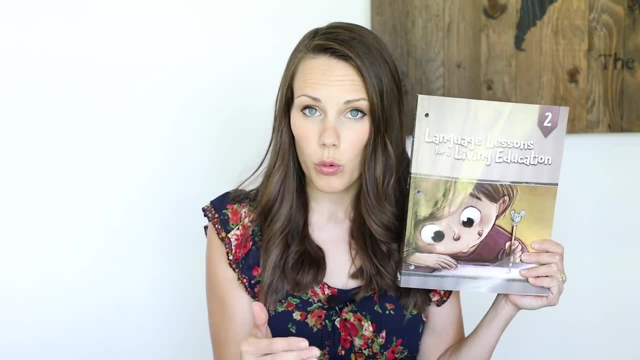 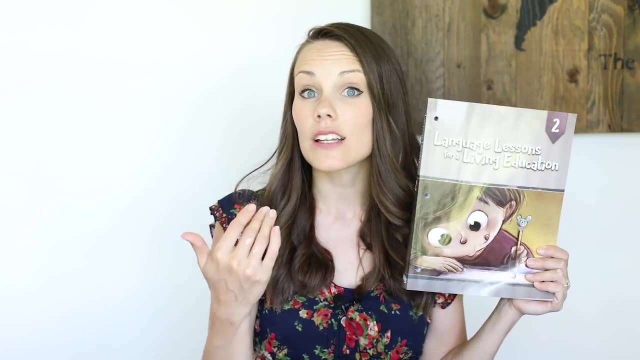 I have really yet to find a program that is geared towards that, because most curriculum is over-the-top comprehensive. That is because parents like me get worried that it's not doing enough and we like things that are in-depth But our kids do not want to get. 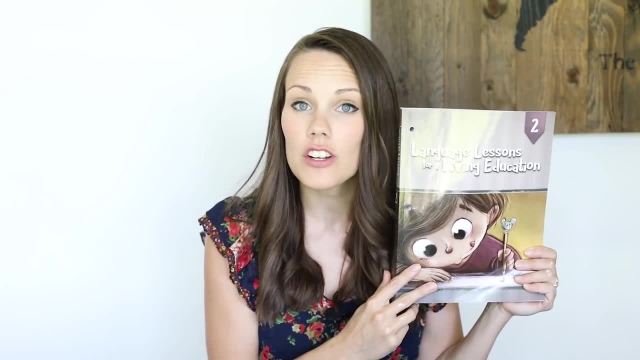 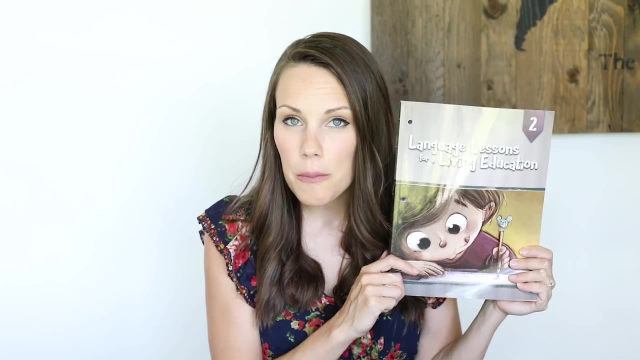 not. Our kids have a natural kind of limitation on how much they can absorb and how much they can retain in a set amount of time, and they have a limitation on their attention spans. So we want to capitalize on that, and the way that this program is set up is to just teach. 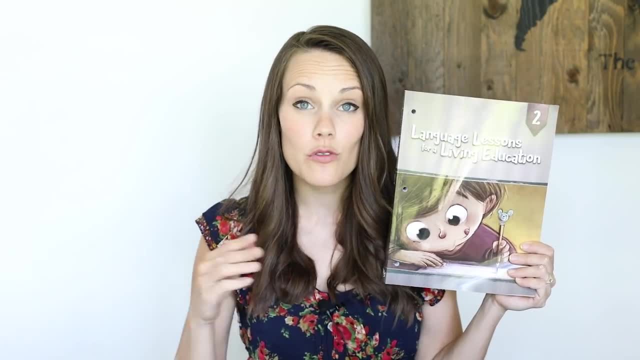 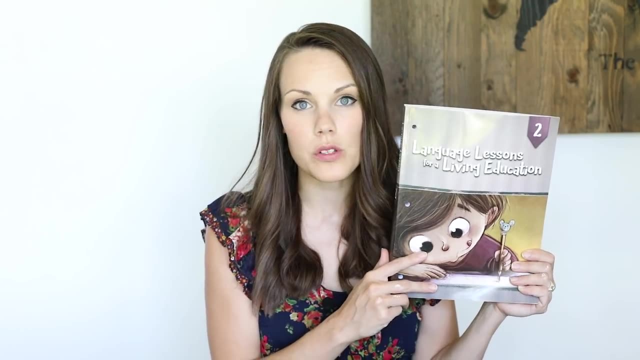 them exactly what they need to know in a short amount of time and move on. That also gives you the flexibility to add in the other things that maybe you use in your home school or you want to use in your home school, like maybe a fantastic spelling. 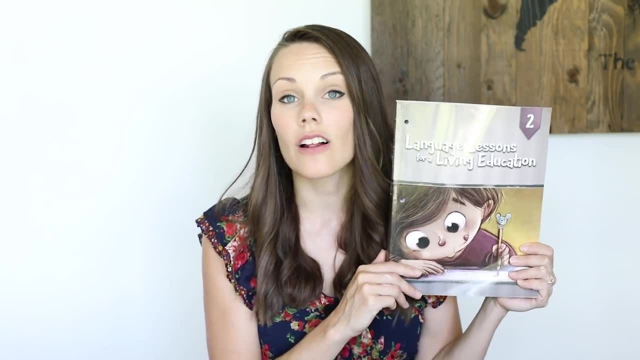 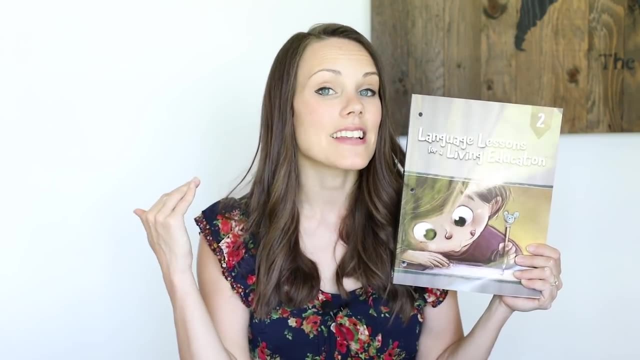 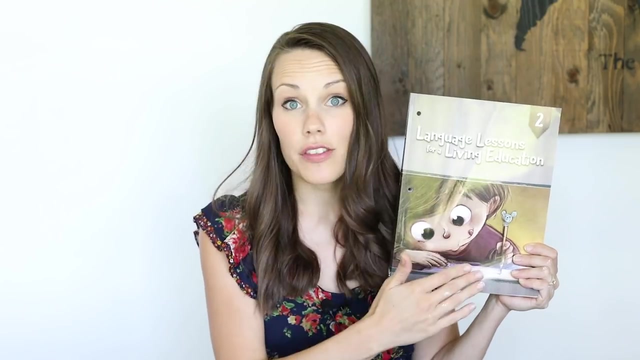 program that you don't want to leave. That's fine. You can do that along with this, because it gives you that flexibility. So it is a comprehensive language arts curriculum. It has everything in here, from reading, writing. it has grammar. it has everything. okay, that. 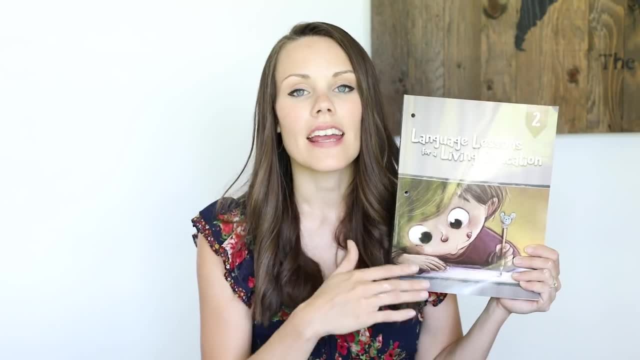 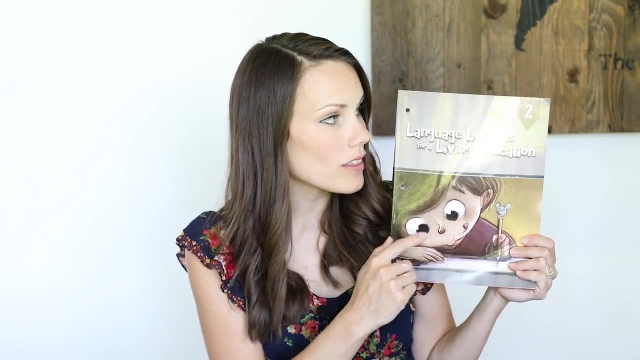 you need Spelling, it's all included. however, it is in a gentle approach that allows you to also adapt it to your family. Right now, Level two is available, and I feel like we need to talk about that because one of the 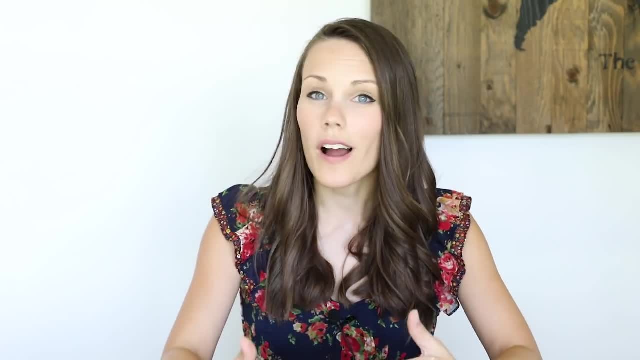 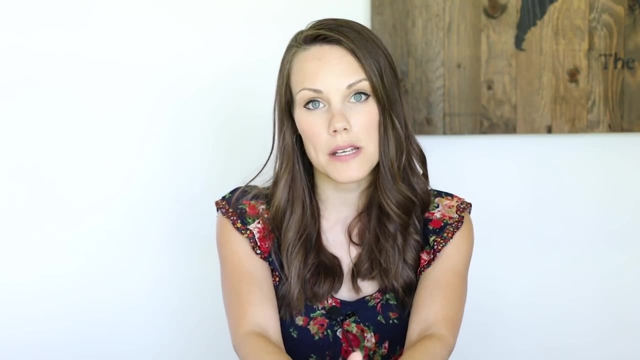 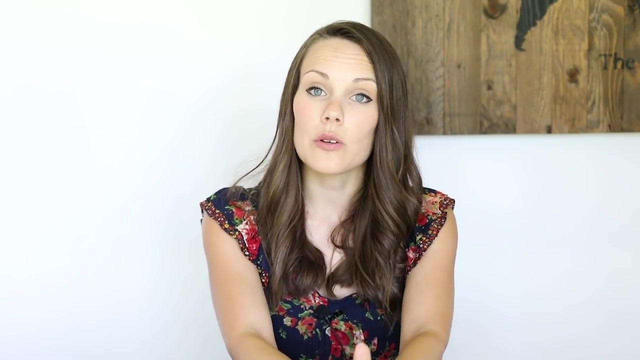 questions that I am getting a lot is: why level two? why not start with level one? Well, let's figure that out. So with master books, they have so much amazing curriculum available that they already had a resource available that kind of takes you in that grade one zone, which is foundations. 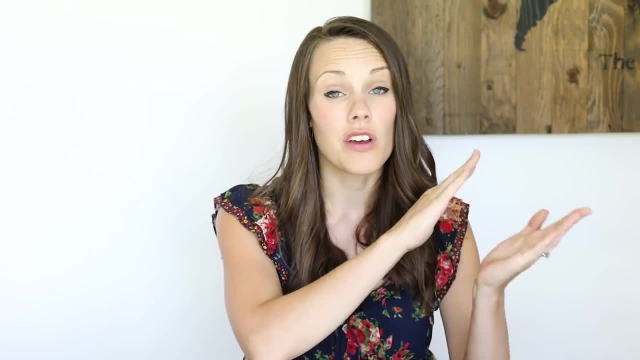 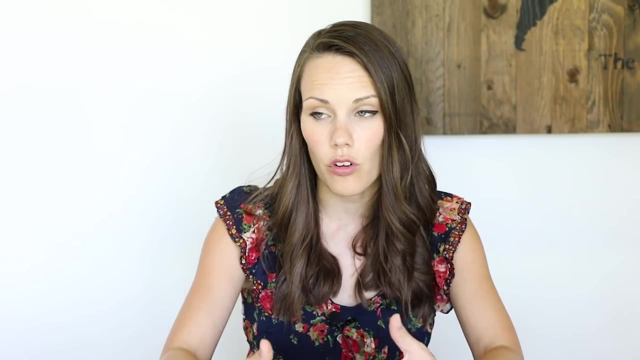 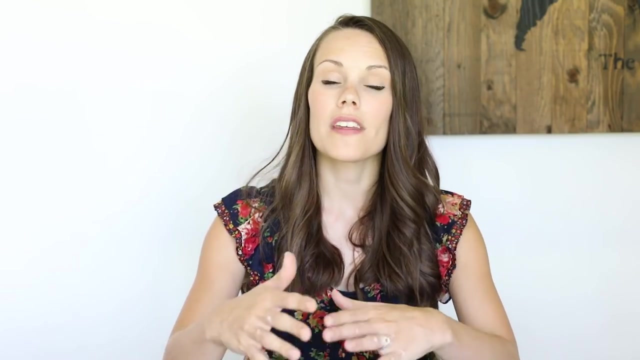 phonics Foundations. phonics teaches you from the basics of letters and sounds all the way to early reading. So they already had a resource available for that level. They also have a later resource that is um elementary Bible and English grammar. So they decided we have this gap in the middle. 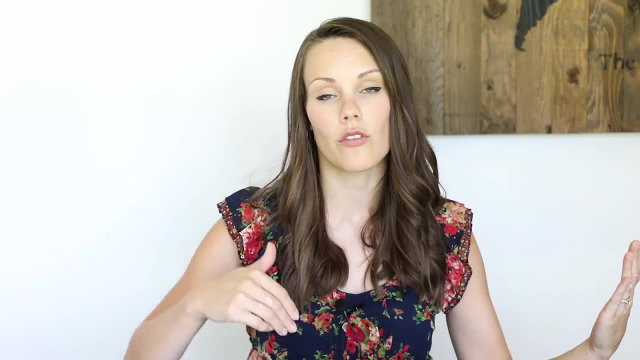 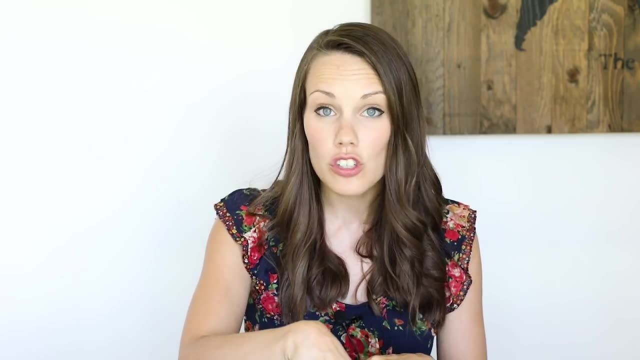 Let's fill this gap first and then we'll go back and we'll do level one and we'll do a level six. So those things are coming, but right now they're filling the gap. So we're starting with level two, Level three is coming out towards the end of summer and then we have level four, which 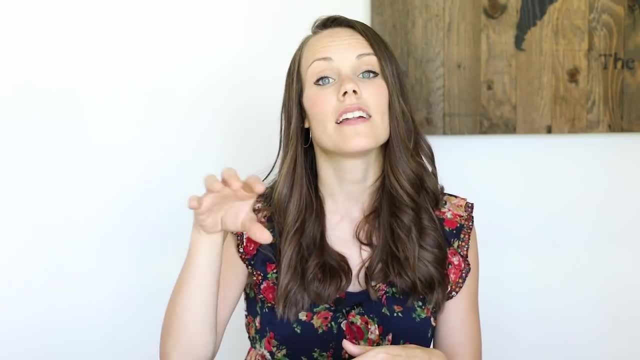 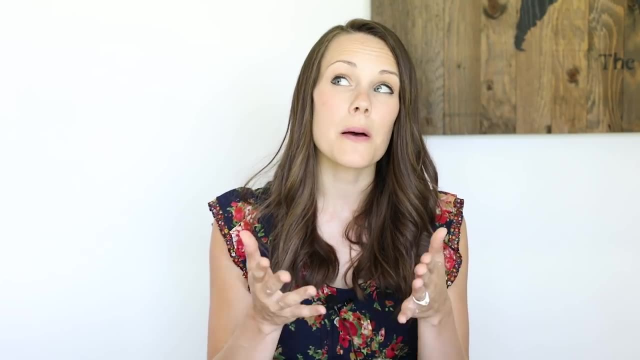 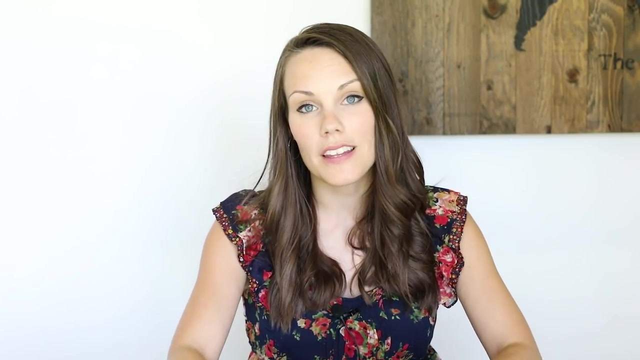 is hopefully coming out. It's coming out around Christmas or the new year and then level five and then we'll reach the either end of that spectrum. So it is coming. Level two is about a grade two level. However, the reason it's leveled is because there is so much flexibility in where kids 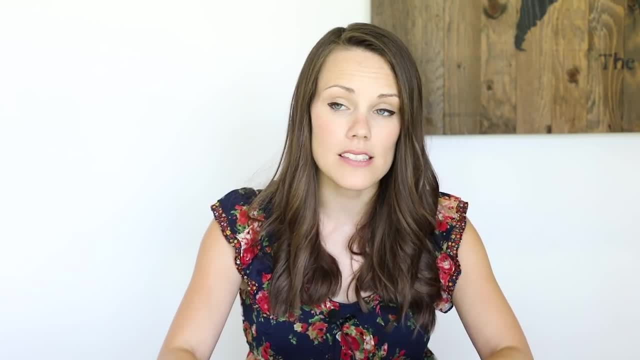 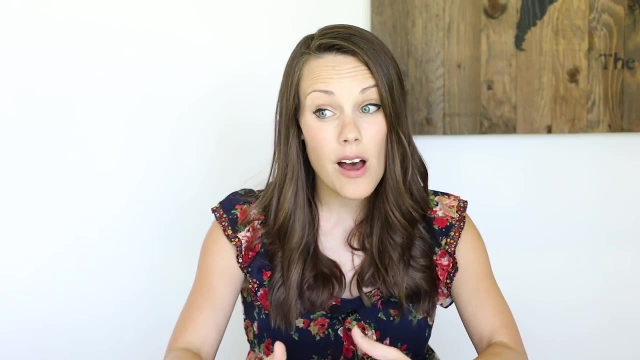 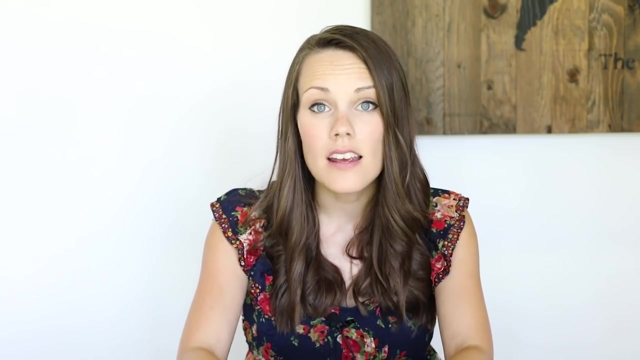 are at at which ages every child develops at their own pace. So some grade two children- this would be too easy for some grade one children- will be ready for this. Some Three or four children could easily do this program. So it is less about the grade and it's more about what's taught and where your child is. 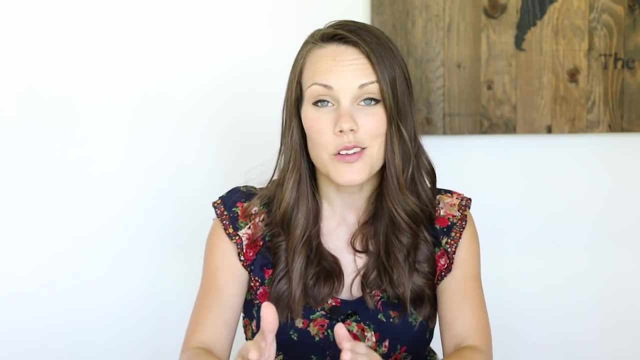 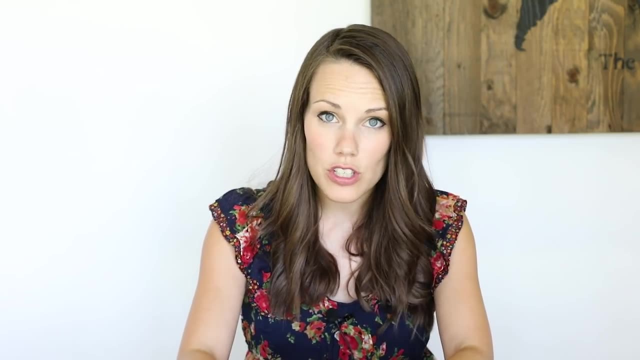 at what kind of gaps they have and where they need to start. So that is how you kind of identify. the best way is to go onto masterbookscom, Take a look, search language lessons for a living education and take a look at the sample. 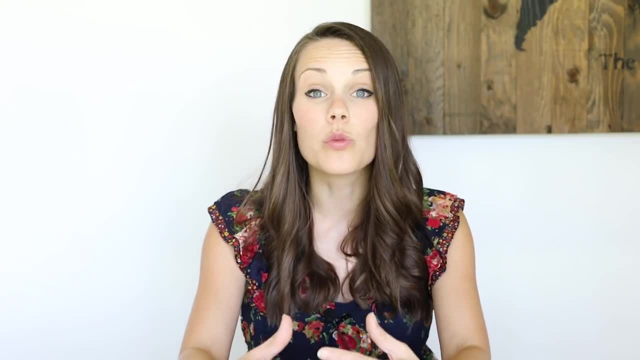 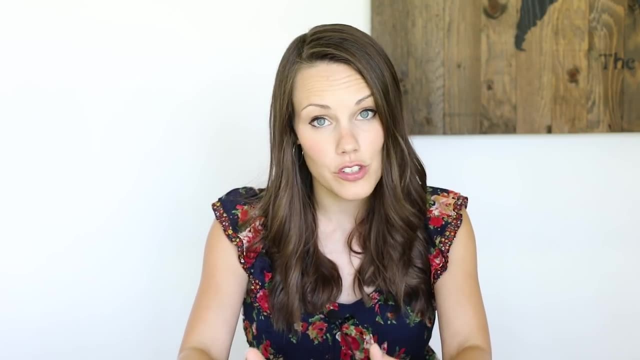 because if you download that sample, do a few things with your kids. that's really going to help you identify if this is going to be too easy, Too hard, Too hard, Or if your child is ready to start with level two. If not, you can always go and order the later levels or wait and level one will be coming. 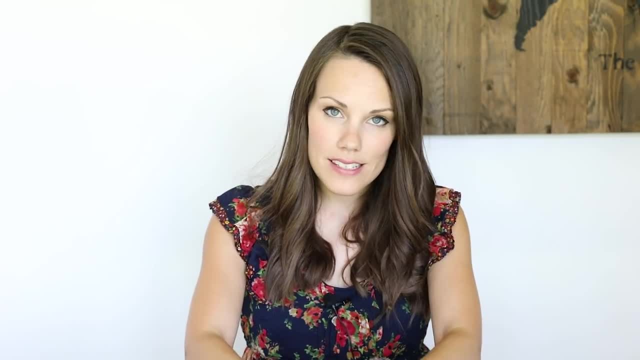 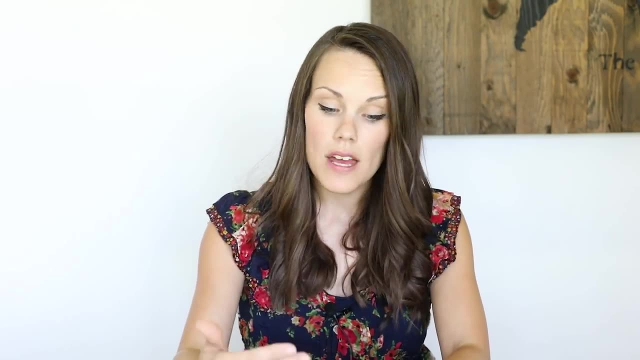 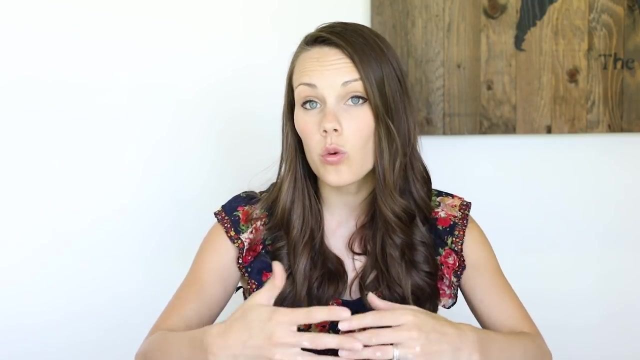 out soon too. So that's placement. The way this is set up is in a five day schedule. Day one, you would do a story or a poem or a Psalm. day two and three: you're starting to go into grammar and writing mechanics. Day four: they're going to create their own story or poem or Psalm. 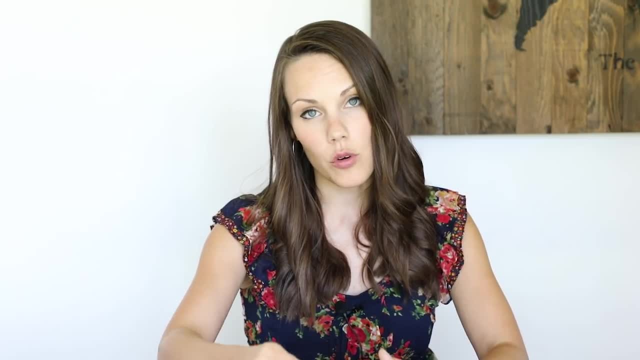 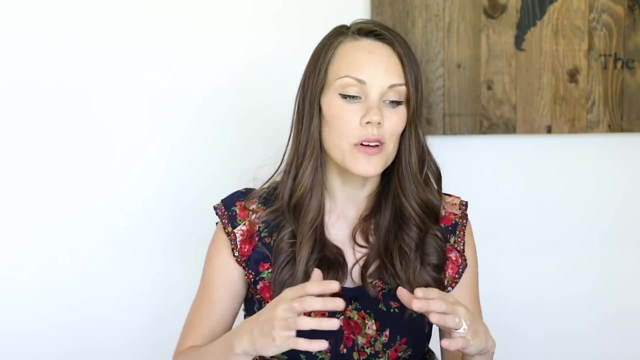 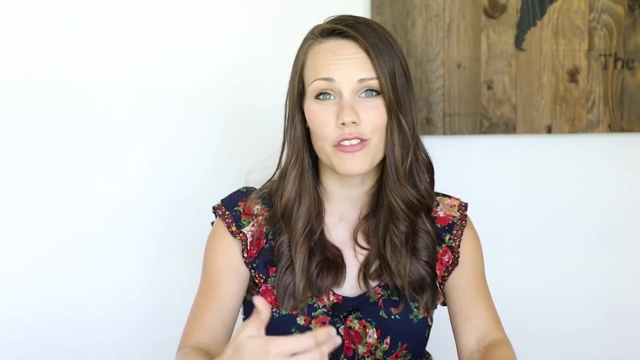 And then Day five is focusing on spelling and vocabulary. So that's kind of the framework of what is in this program. But really I know that the very best way for you guys to get a grasp of what it is would be for you to come over have some coffee. take a look through the book. 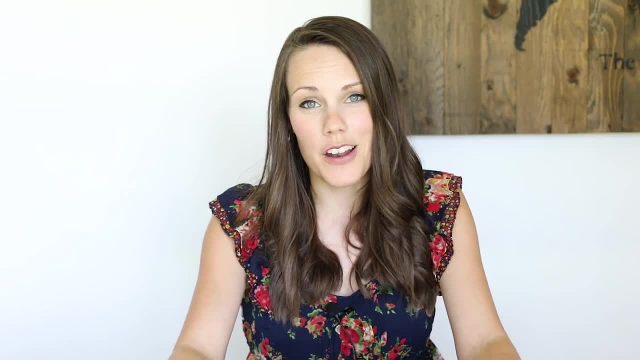 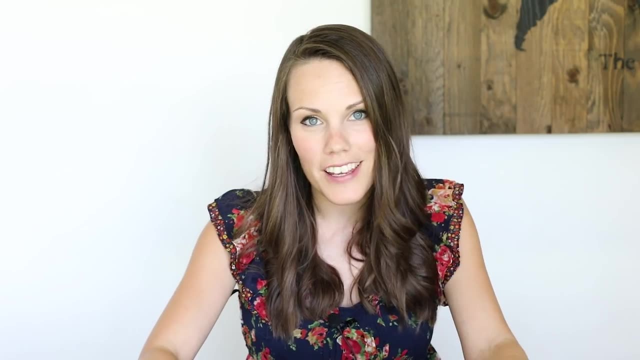 Now I live in Northern Canada, so that may not be possible for a lot of you. However, I can make it possible for you by giving you the next best thing, which is a close up. So let's take a look inside this curriculum and let's talk about what is inside. 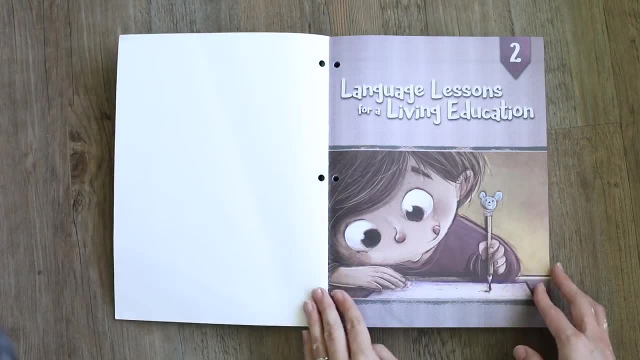 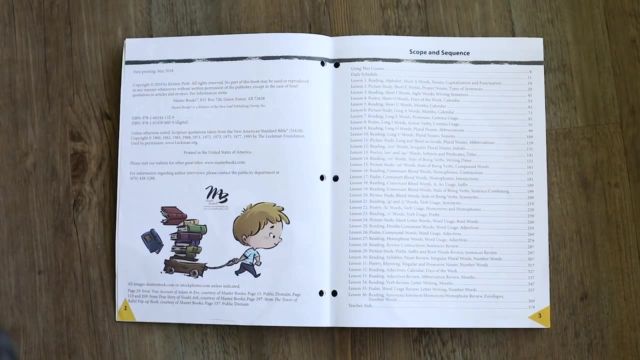 All right. So the first thing you're going to notice when you open it up is the scope and sequence, And this kind of gives you an idea of the different things that are covered throughout the year. It goes into how to use the course. 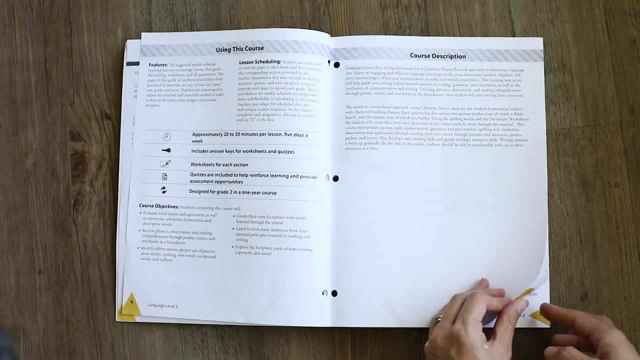 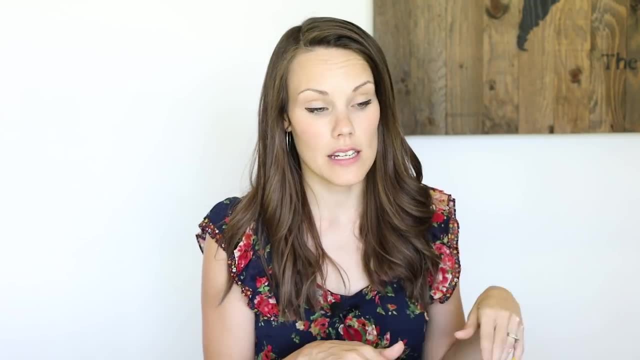 So the features. it tells you it takes about 20 to 30 minutes a lesson. It really. I mean maybe could as you get farther along in the program, but I find that 15 minutes seems to be the most that it takes us. 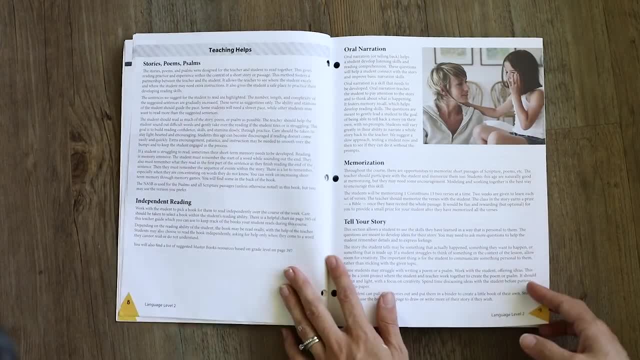 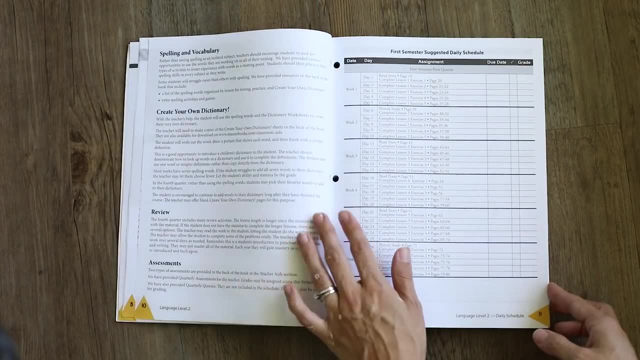 Even with drawing a picture. So there's teaching help. So this would be where you go if you wanted to understand the different elements of the program, like stories, poems and Psalms, how they're used. independent reading- oral narration. 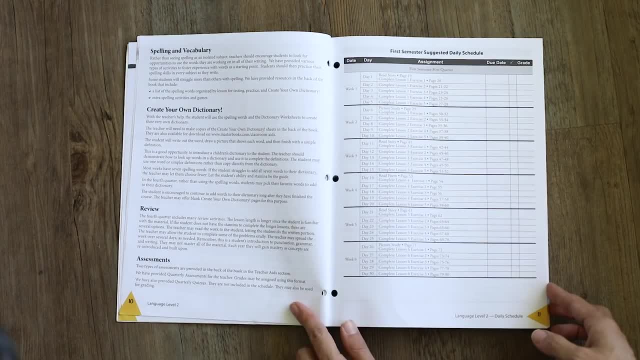 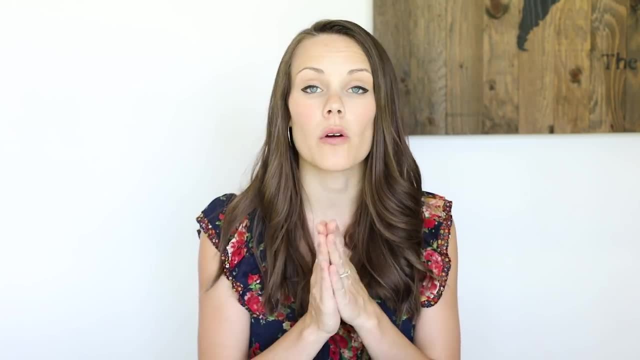 memorization and the tell your story, the spelling and vocabulary, create your own dictionary. And then there's also reviews and assessments built into the back that you don't have to use, but are included if you live in a state or province where it's required in order to 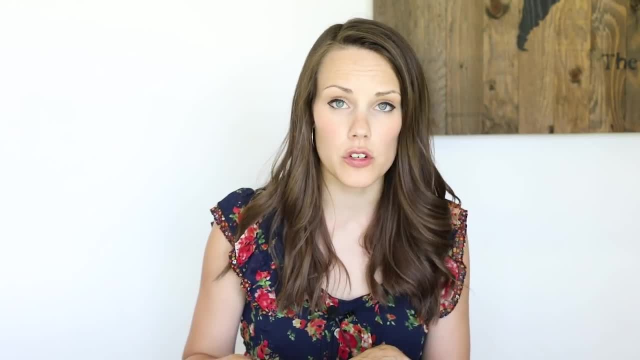 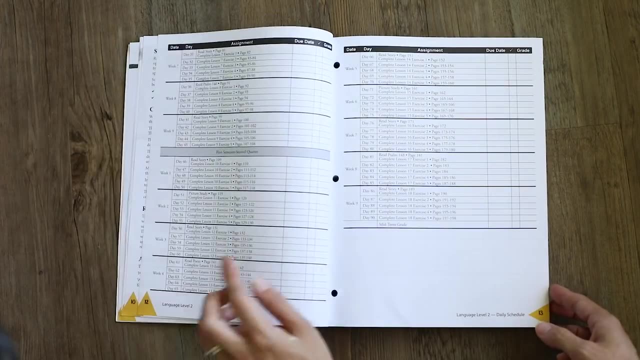 have something to grade and report. Now all of Masterbook's curriculum comes with a very easy daily schedule in the very beginning that you can check, you can grade if you need to keep track of where you're at, and it just tells you exactly which pages to do on which day. 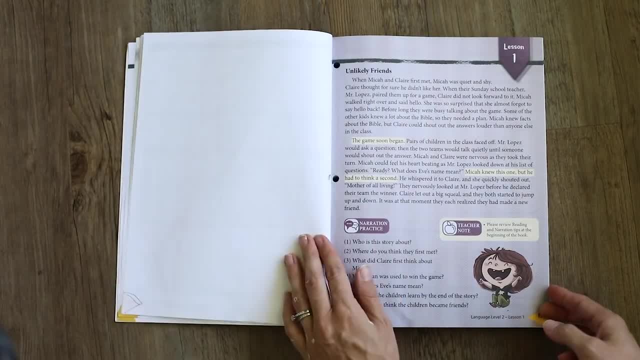 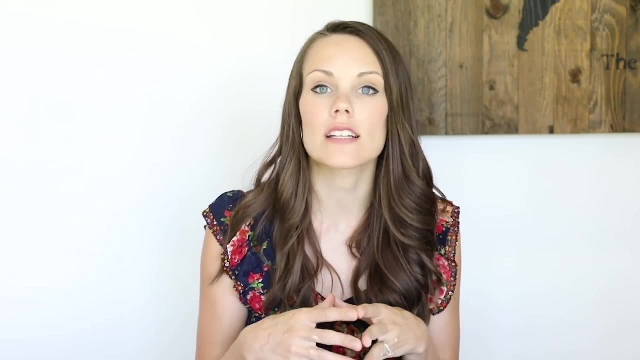 So now we're at lesson one. Just to give you an idea, I'm going to show you at the beginning of the book and the end of the book what the lessons look like, and you'll see the same frame repeated. however, you're going to see how they advance. 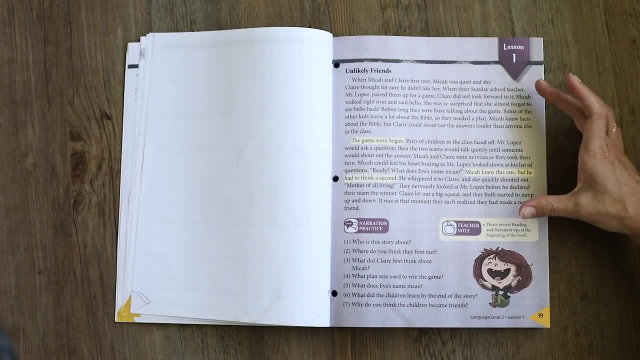 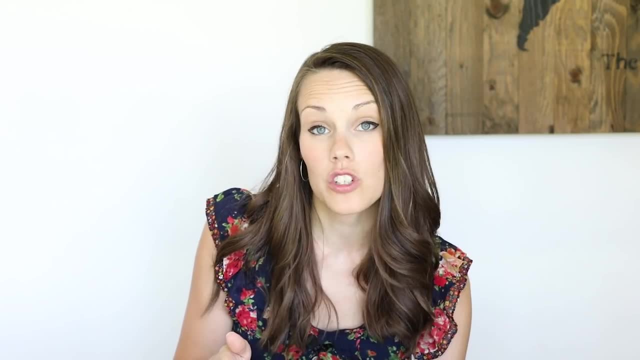 So in the first week- you're day one- You're going to read this story and you'll notice that there's some highlighted portions here, and these are actually things that your kids get to read along with you, which is really a unique aspect to this program, because you read some of the story which draws them. 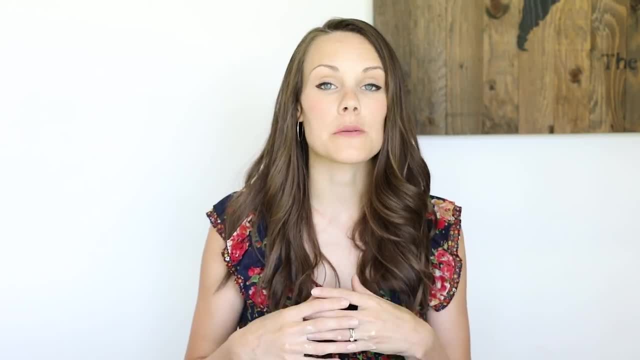 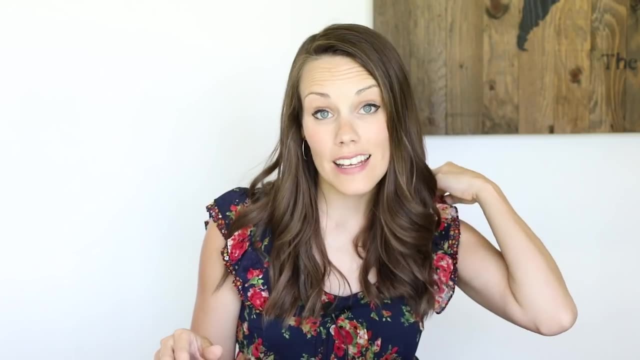 in and then they get to read part of the story which keeps them engaged in it. So there's narration practice. there's little notes to the teacher throughout the program. however, it is written to the child so you really don't need to even think about it. 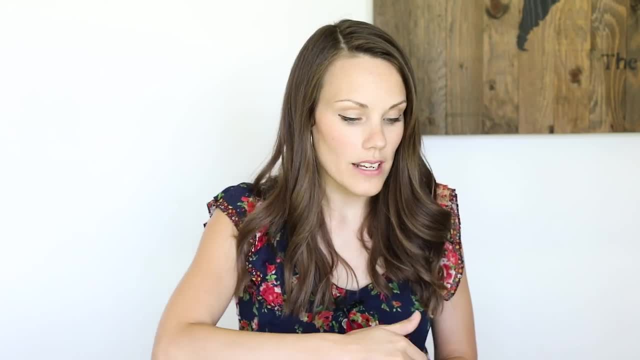 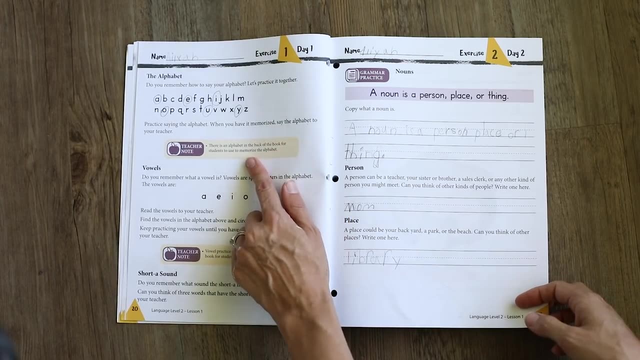 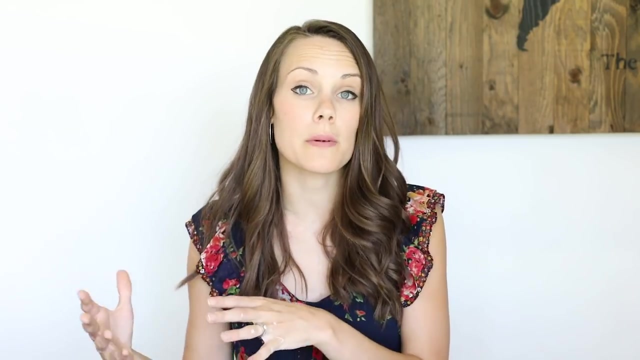 You just read and go. The other thing you're going to do on day one is a worksheet and it starts off very simply with the alphabet. and it's not that we're learning the alphabet in our letters and sounds in this program. It's just to give us a frame to get all the kids on the same page before we begin. 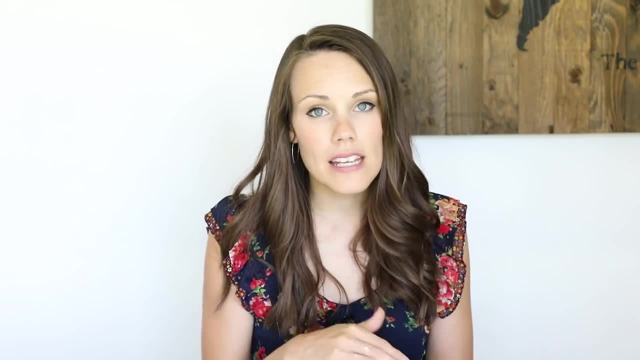 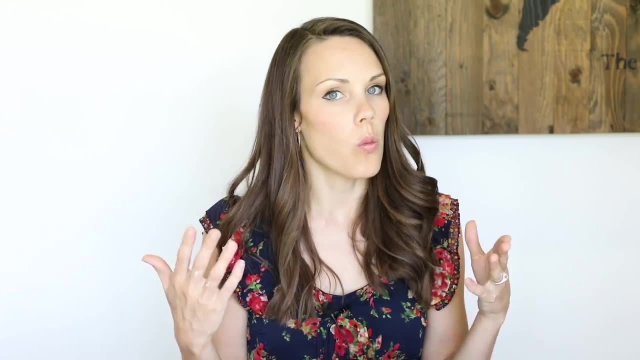 There's even more alphabet practice sheets in the back, because there's some kids that maybe need some more help with writing, or there's some kids that maybe just need a reinforcement. What are your vowels? What are the long and short vowels? What are the short sounds of them? 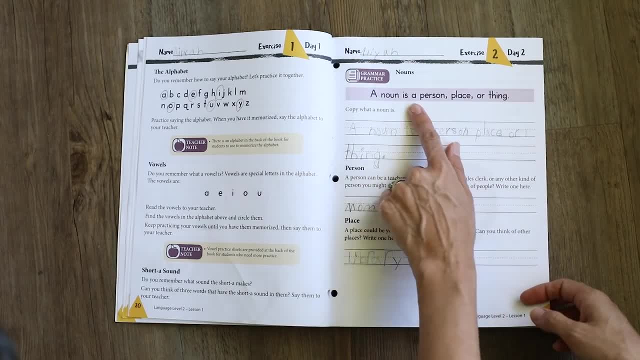 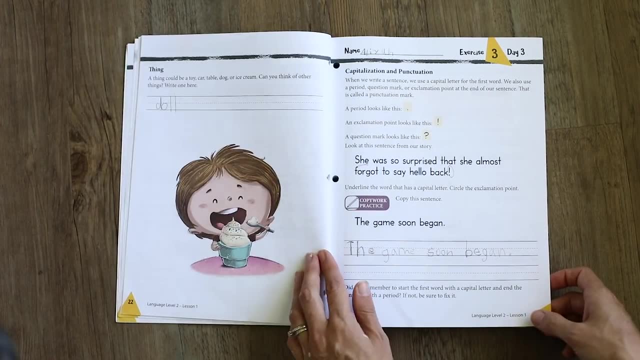 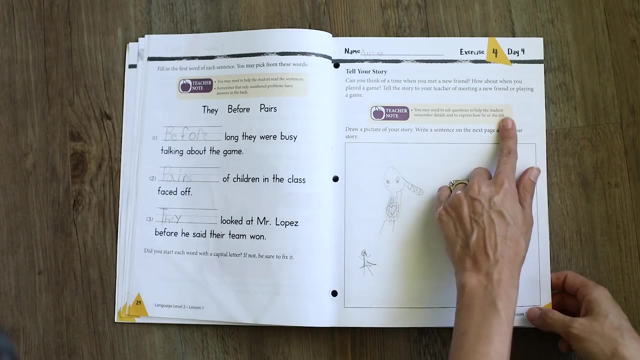 So we start with just a really simple review. Then, day two, you're learning some grammar, so a noun, and they're copying. Day three, they're going into capitalization and punctuation. Day four, they get to tell a story, and this is just such a unique aspect of the program. 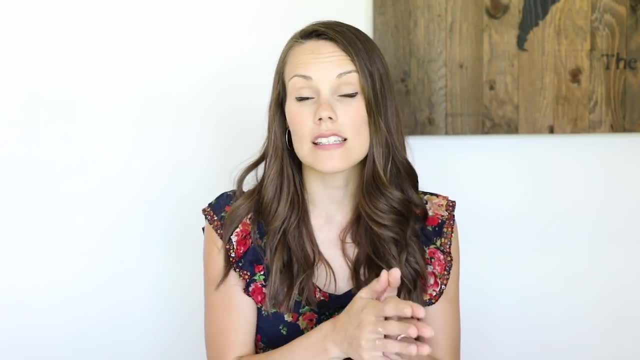 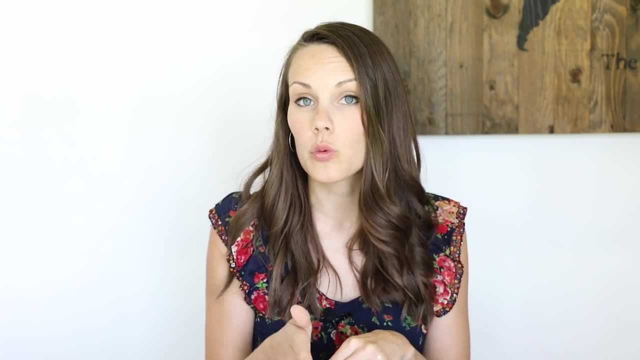 because you can use it so many different ways. You could have your kids narrate to you. You could write it out for them and then have them write down on the next page. They have to write a sentence about their picture. You could write it on a board for them, the sentence they want to say, and then they can. 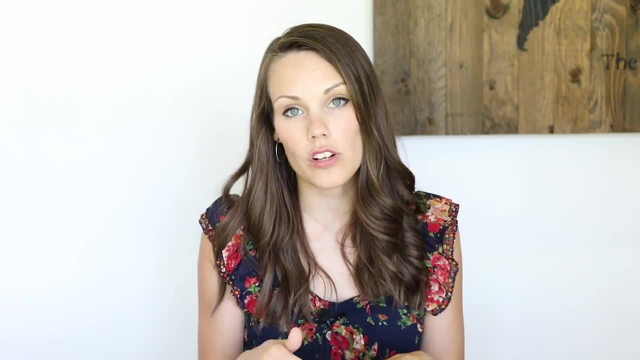 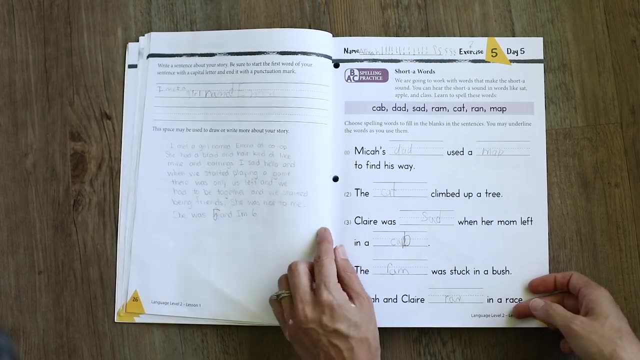 copy it, or you can just coach them through the spelling of the words as they're writing. So that gives them some prompts. and then they draw a picture, and then they're going to write about their story, And in the beginning of the program it starts with just one sentence. 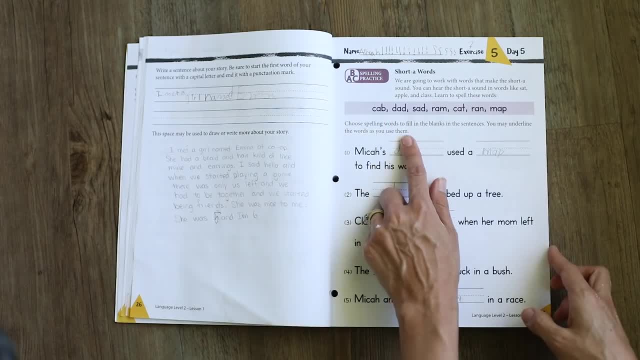 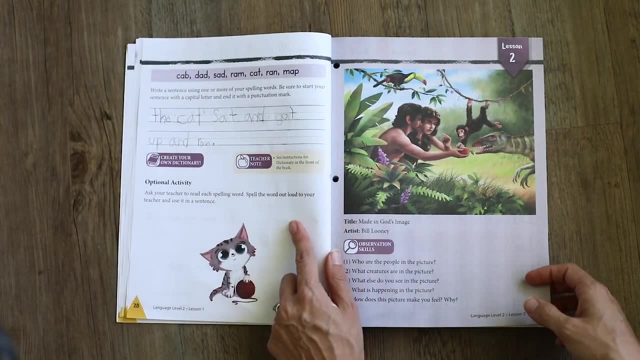 On day five there is spelling. Now this is spelling kind of worksheet. Here's your words at the top. There are spelling lists in the back If you'd like to go more in depth on these and work on them. every day there's spelling. 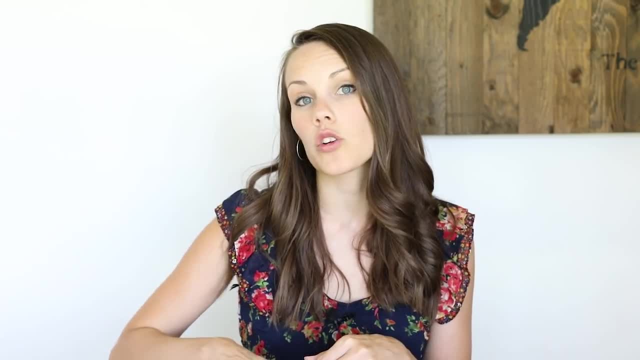 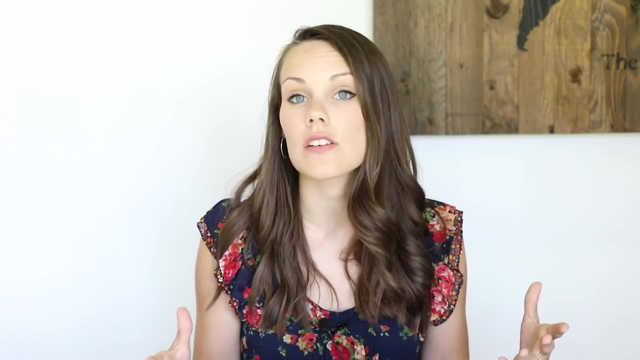 activities in the back that I'll show you. But basically these are the words that you could use, or you could just do these worksheets for spelling practice and use, like I said, your own spelling program or anything else that you want to add to it. 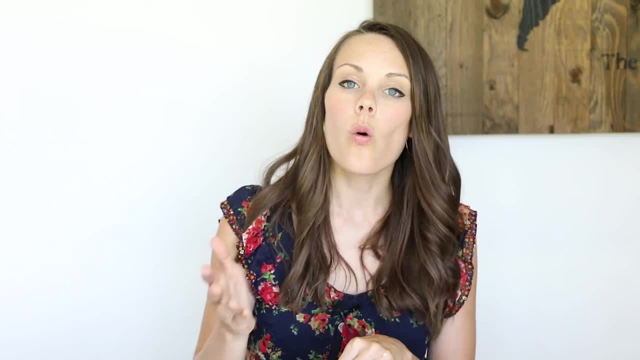 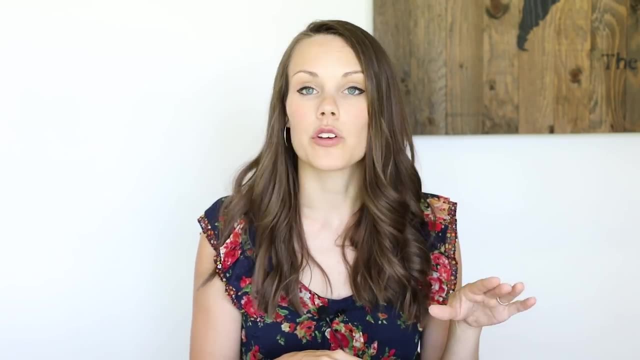 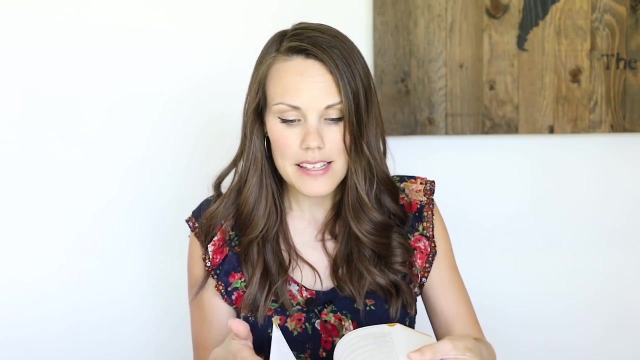 So there's flexibility to use the spelling within here or to add your own routine or whatever you're using that you love. So that lays out your first week. Now, if we flip forward to week three, Week 36, the very last week in the program, that's going to give you an idea of where 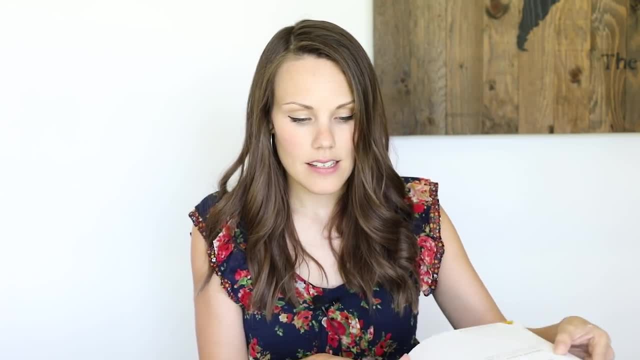 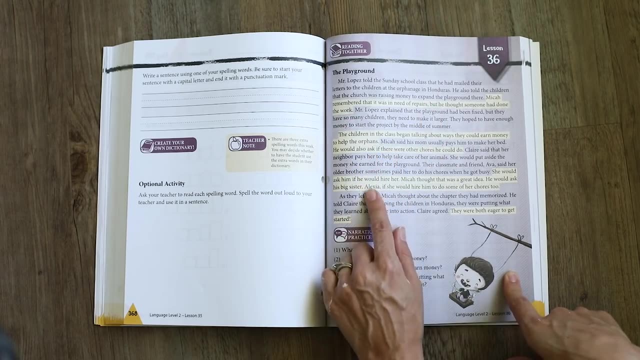 the program takes you to. So by the end their reading together is more. They're reading more with you. You can see there's quite a bit more highlighted sections here, So they're reading the story. and then there's observation skills and they have to write. 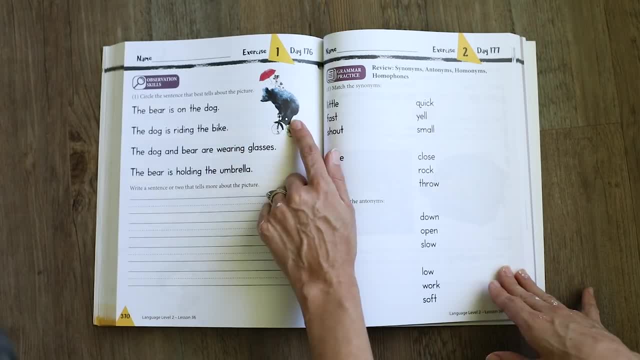 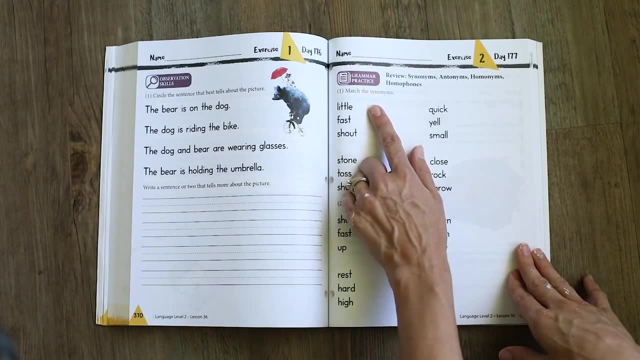 a sentence or two as well. So that is day one. So we're getting more advanced in the amount of writing we're requiring, in our observation skills and in our reading. On day two, there's grammar practice, and it's going into much more depth. 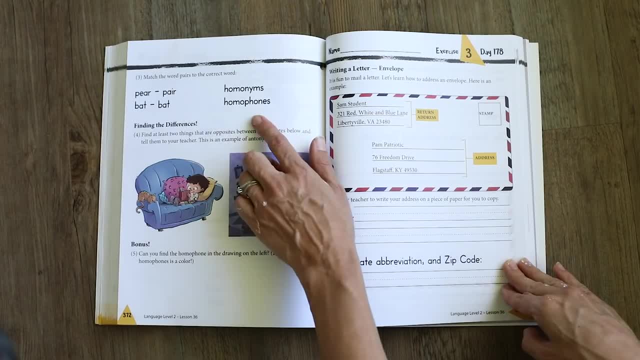 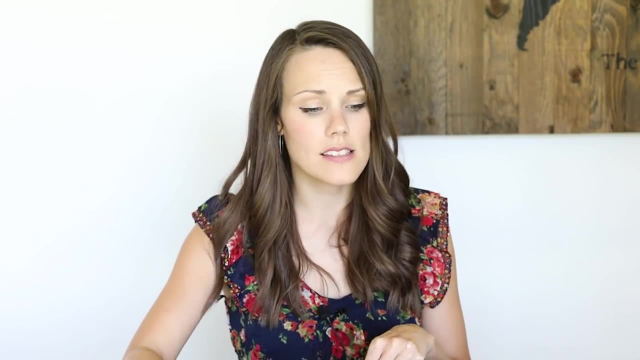 As far as grammar, it's very, very comprehensive. There's nothing you need to supplement with this. Synonyms, antonyms, homonyms, I mean you guys, my grade four hardly knows that stuff. So this is in-depth, comprehensive program. 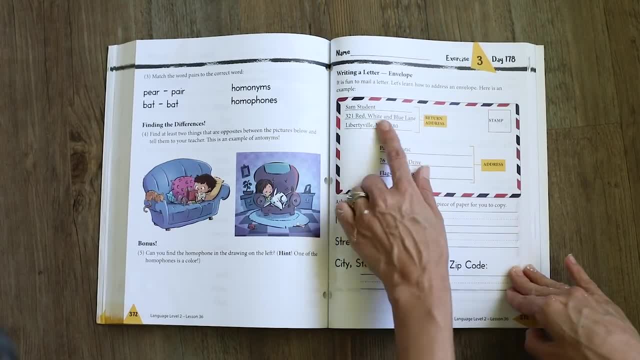 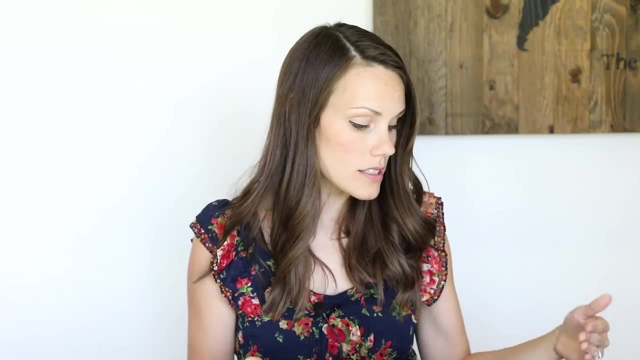 Day three: they are learning how to address and write on an envelope, the proper places and positioning And if you look here, it says day 173.. So the week previous they wrote a letter And so they can mail their letter and actually practice that as well. 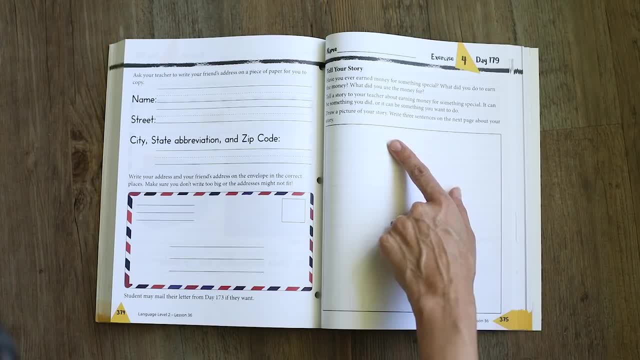 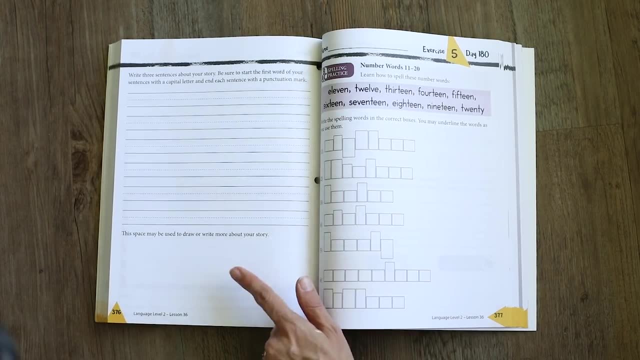 Day four. you're telling a story. It gives you some prompts, but on the next page, instead of one sentences, they're now writing three sentences. So you can see how we are. we're we're adapting, we're growing. it's getting harder, it's getting. 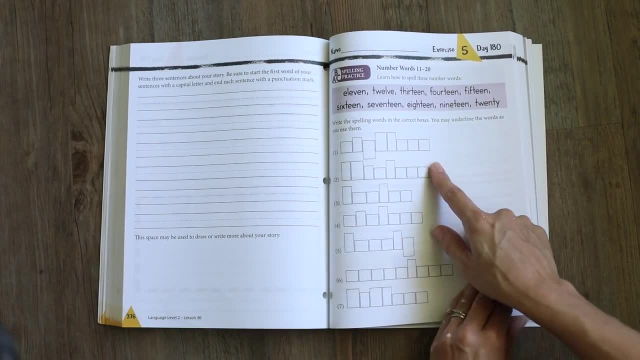 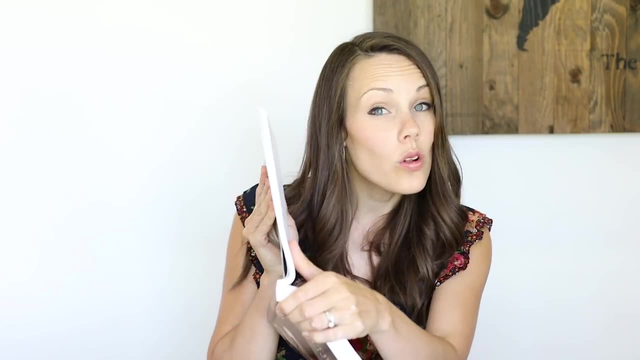 more complicated, And then our spelling practice, our words, are a lot bigger as well. So that's kind of where it starts and where it takes you to, but I don't know if you can see here, there's a whole lot of book left after you're done all of that. 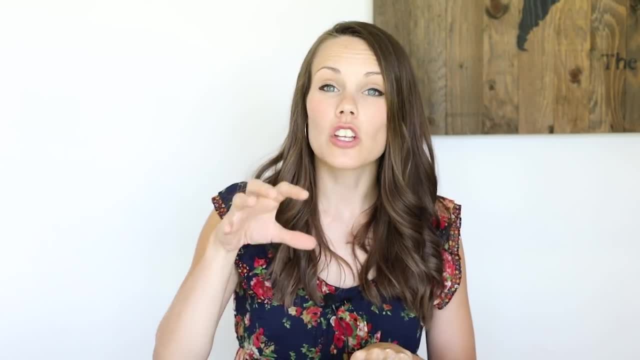 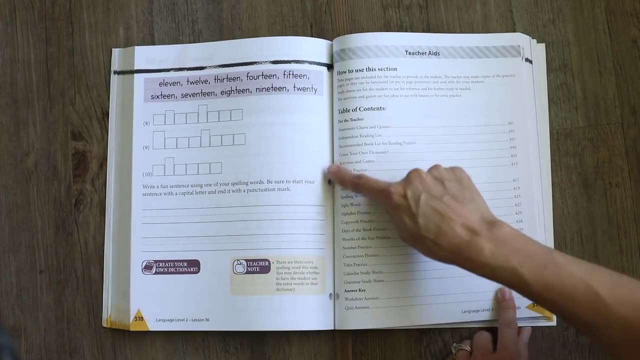 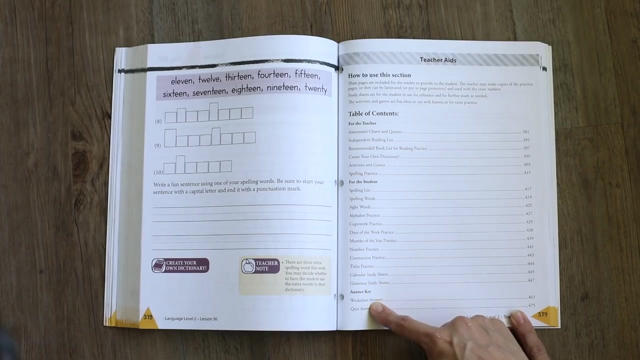 And this back section is all of your teacher aides that you can use to adapt this program to your child, that you can use to give them extra practice, that you can use to give you more ideas. Everything that you need is in the back. So back here we have assessments and quizzes. we have here- this is a assessment chart- 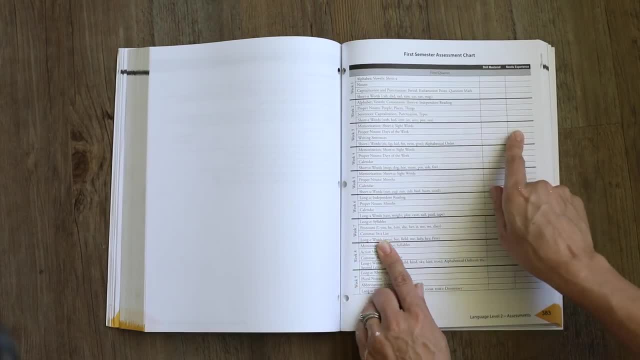 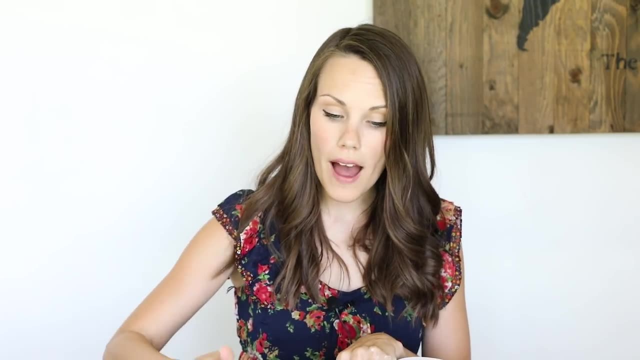 So this is really helpful for the actual um, the actual things that are being taught. This is where you can check off what is mastered and what they still need experience in, And if you go back and you look after a quarter, there's some things we still need more practice. 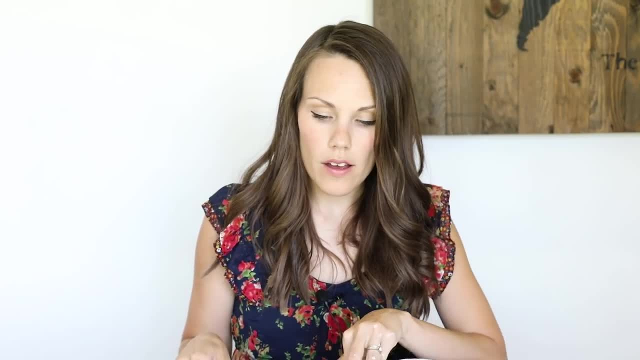 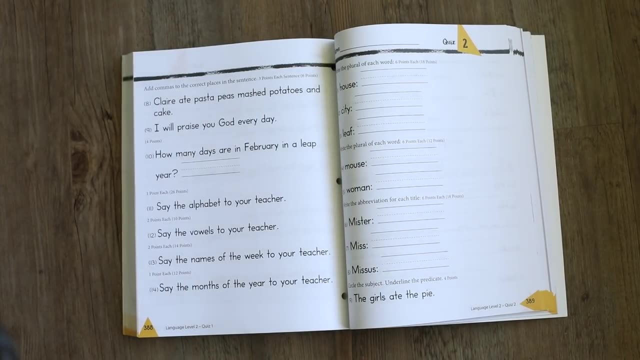 There's additional practice sheets back here as well. So if we go up here, these are, these are quizzes, So again, you don't have to use them, but if you felt like you needed to or you wanted some way to assess your child's progress, you could. there is a reading book list there. 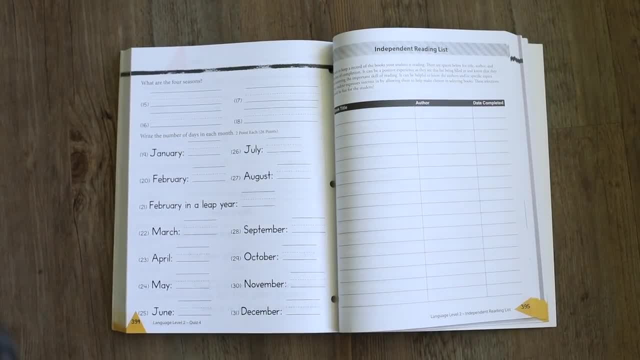 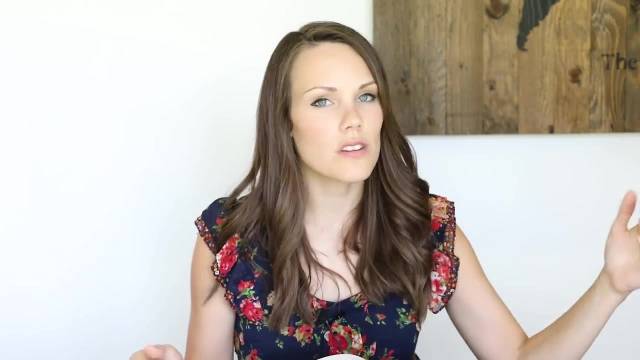 So it will prompt you to do independent reading. There is, right here, Some recommended book lists. These are master book titles that could be used for each grade, or you can go to the library and choose your favorite title, or let your kids pick their own readers, or however you. 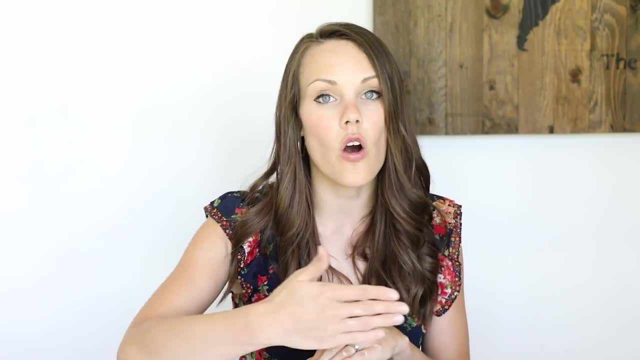 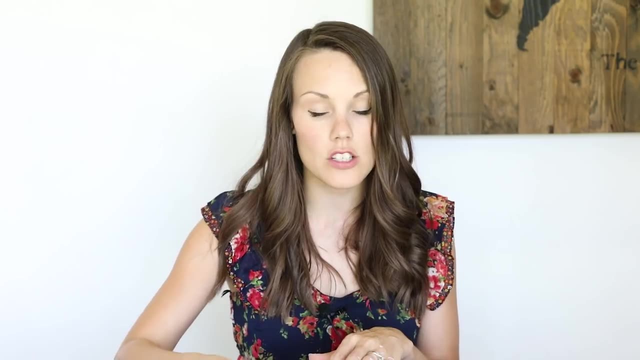 want to do it, But it does encourage you to do independent reading on top of this. They should be reading more than just you know those few sentences once a week. So it does prompt you throughout the week to do independent reading, and there's a place. 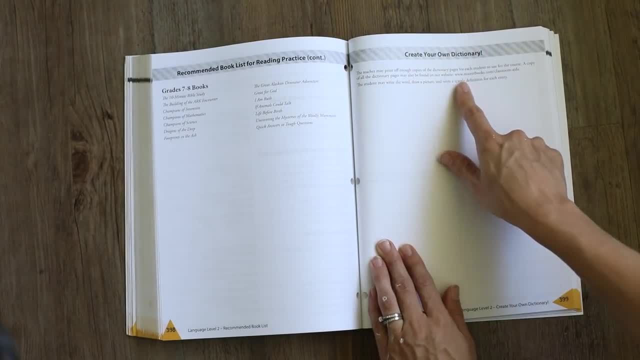 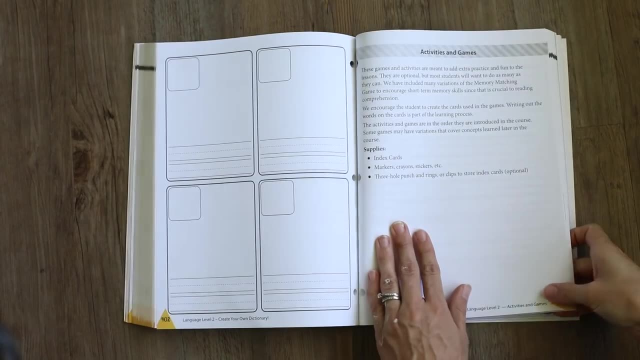 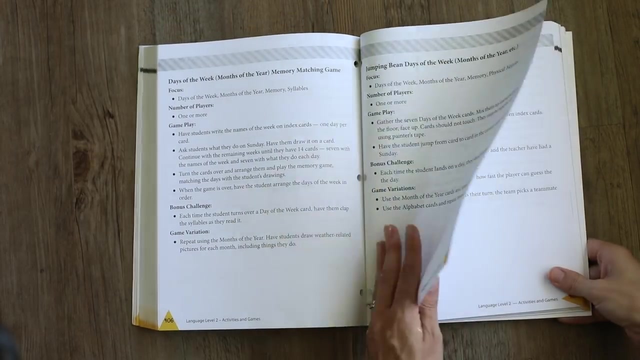 for you to keep track of that. There is a create your own dictionary section so you would photocopy this, cut them out and your kids are going to be throughout the year creating a dictionary. and then there's an entire section of activities and games that you can do to expand on the lessons for 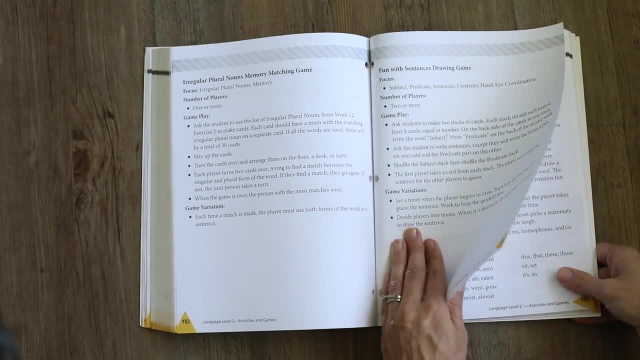 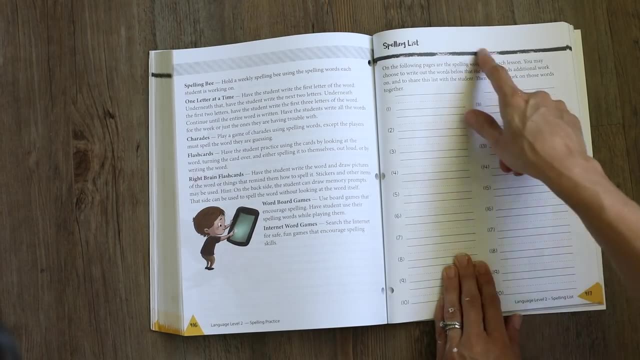 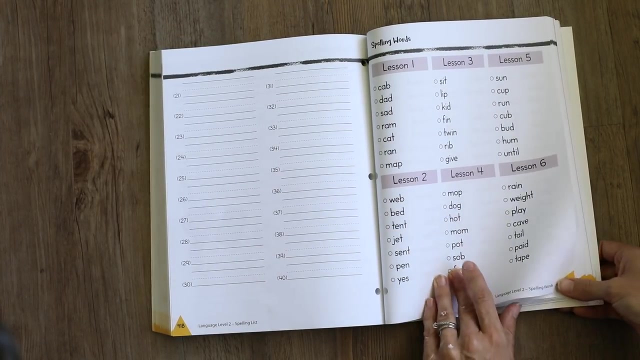 spelling and for reinforcement. There's spelling list. Again, you can use this in so many different ways. It's just an additional resource and then all your spelling words for the program are listed here as well, by week. So if you want to use this, you would look at your spelling list, you would do your spelling. 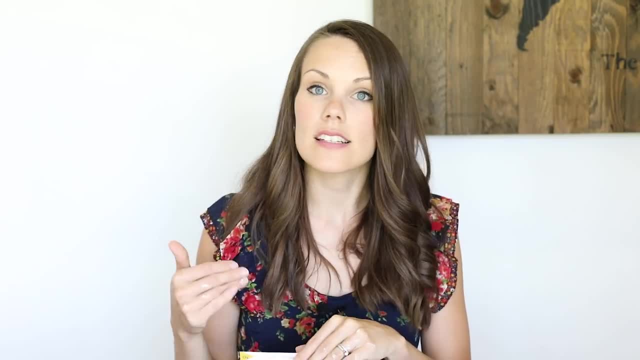 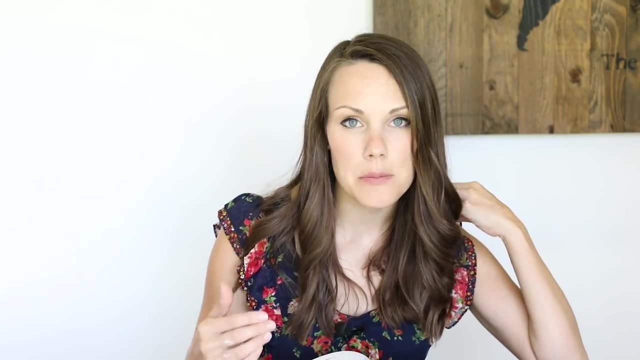 worksheet, maybe throughout the week, and you would have your kids be writing these down and perhaps test them on it, or you can do it a totally different way. So there's so many ways that you can adapt and tweak this program for your homeschool and your child's. 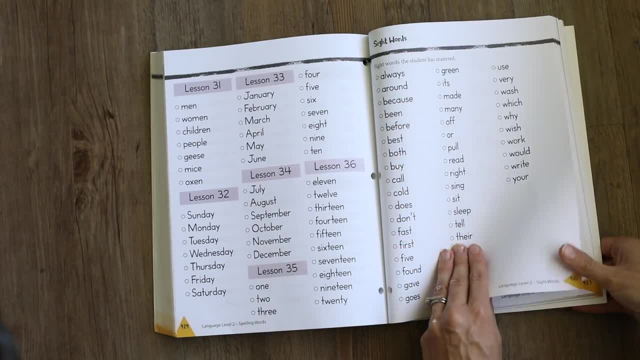 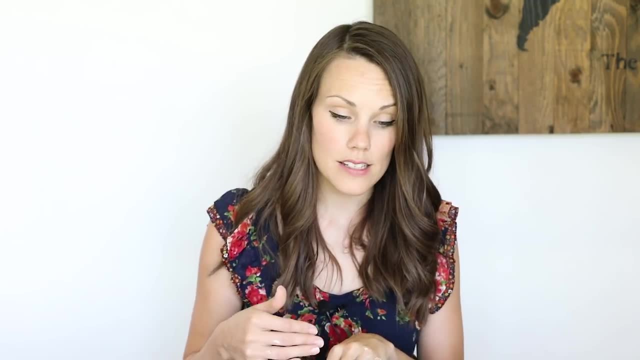 There's also a list of sight words that you're going to want to try to work through with your kids. They're going to be words that they're going to see and they are going to want to master throughout the year. So you're going to keep track of where they're at. 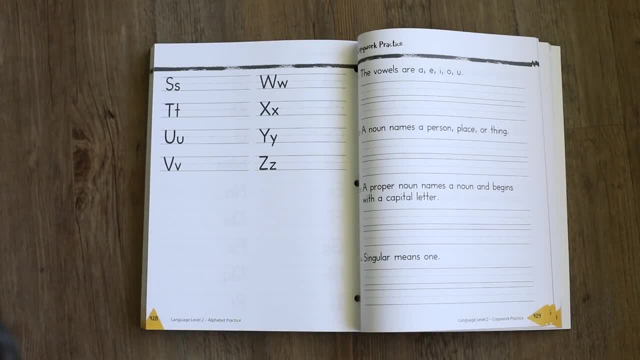 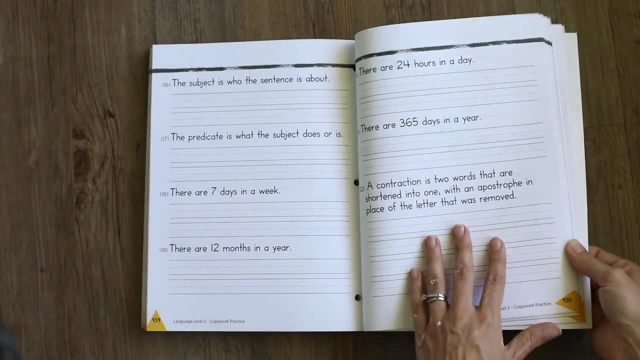 Now back here we have an entire section just for copy work practice And the reason that they included this is so that if your child is struggling with something, you can photocopy one of these and as they copy it, they're going to be reinforcing. 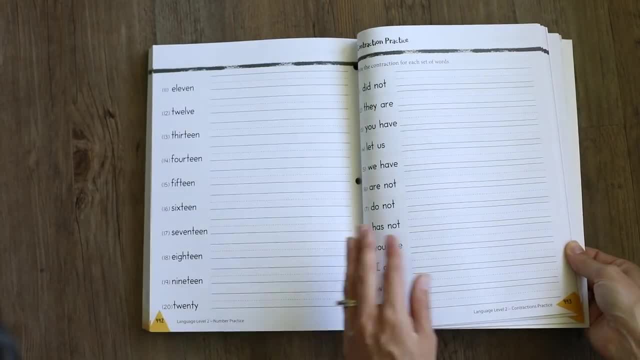 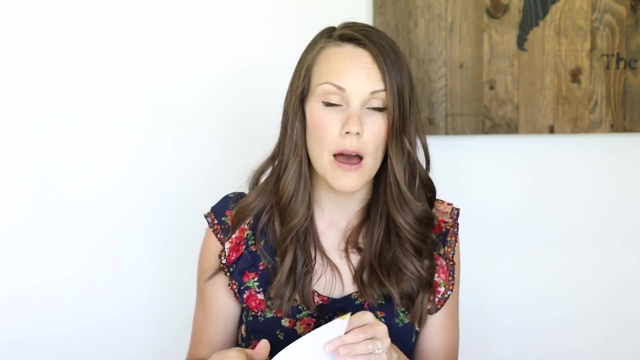 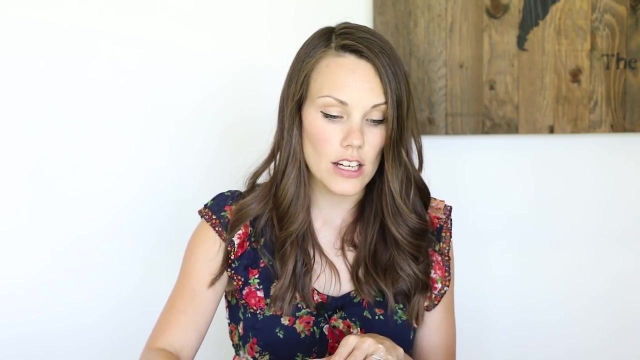 the principle that they're struggling with. So, for example, if they're struggling with remembering what a verb is, then writing it out is going to help them remember it. An action verb tells what is happening in a sentence, So there's a whole bunch of extra copy work sheets in the back for abbreviations and contractions. 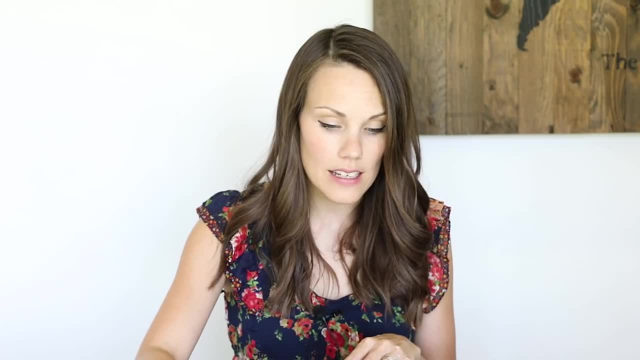 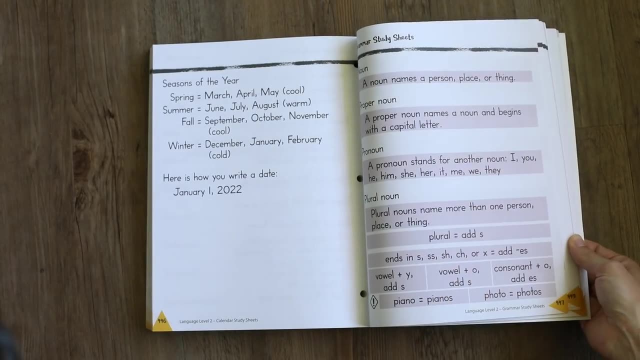 just to give them that. Okay, Give them that extra practice if they need it. And there's also a whole bunch of study sheets, which is really unique. You could tear these out. They're all. the pages are perforated. You could tear them out or put it in a binder and have your child laminate it. 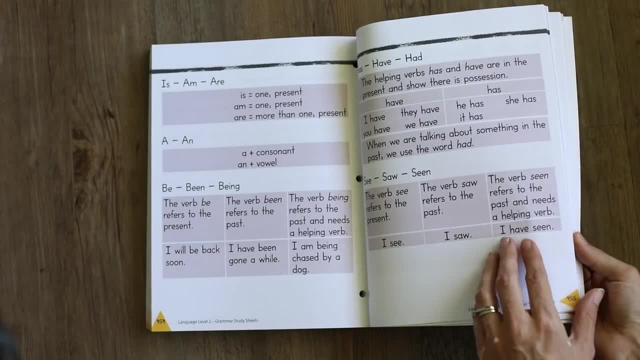 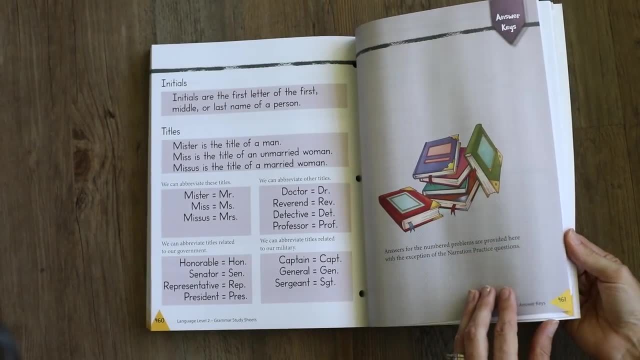 So they're kind of like little cheat sheets that they can refer to throughout the year if they're struggling with something. And then the very last section is an answer key. And this answer key is just purely for you. If you need to mark and grade, you can. 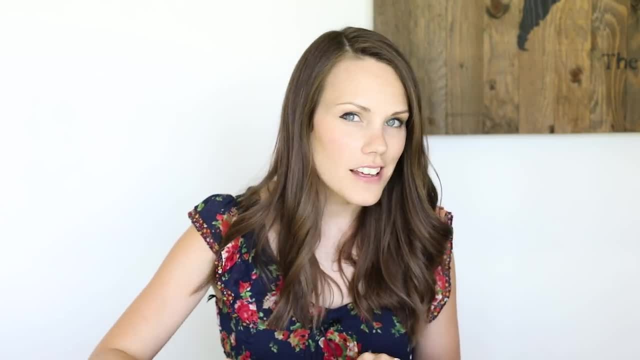 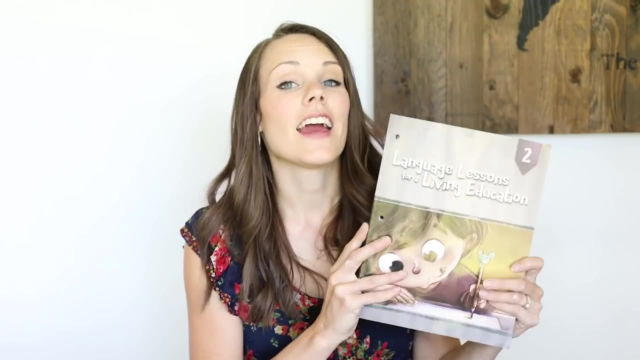 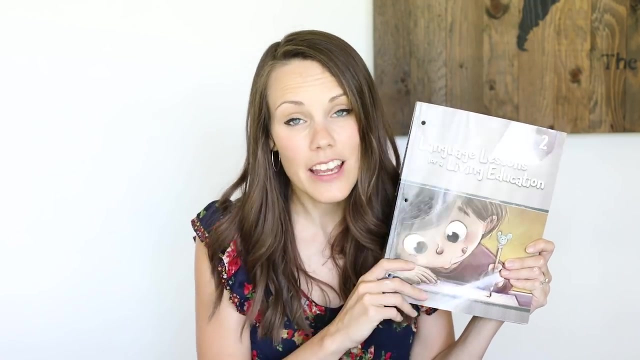 But also, if you aren't a hundred percent sure on what you're going to do with your child, you're going to have to figure out what the answer to that grammar question is. You can find it back here in the answer key. So, as you can see, it is a very comprehensive, full and and fantastic language arts program. 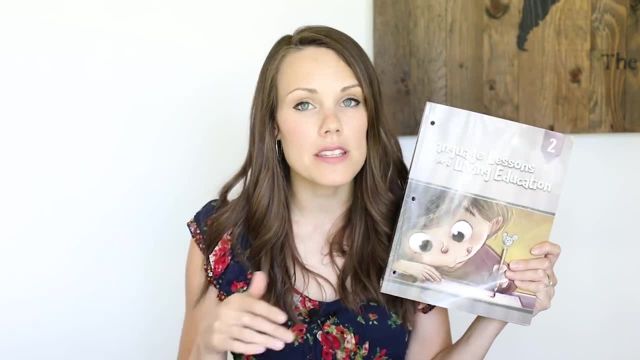 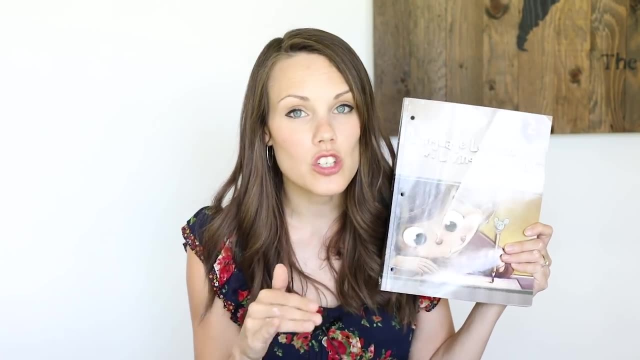 that you can use together with your kids. You could adopt this and use this with multiple kids at the same time. You could use this for a grade three or four. You can use this for a grade one or two. Go check out the sample pages. 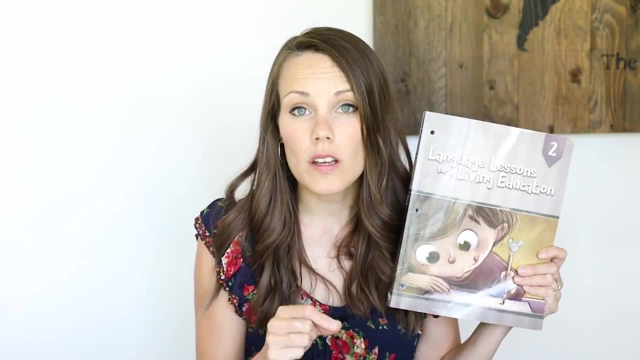 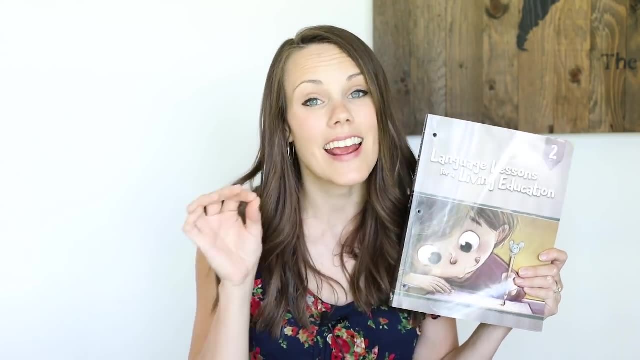 That's going to give you Best idea. And you guys go and join the moms of master books group on Facebook because there's always new resources and questions being asked and answered. that also might give you additional insight into where to place your child when the new levels are coming out and any additional 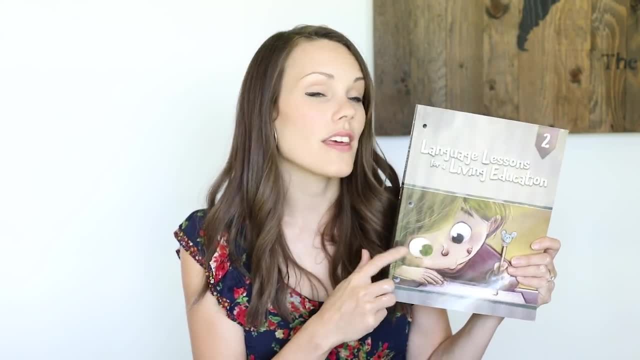 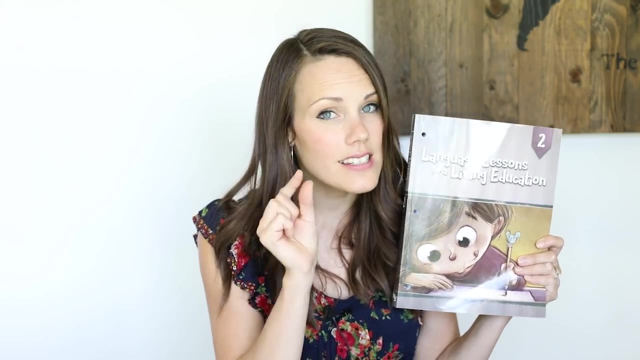 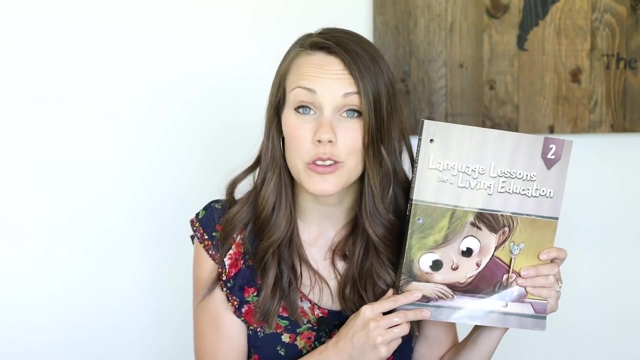 resources that are being added to the program. So there you have it: affordable, comprehensive and yet short enough that it's not overwhelming. It's easy to add to any homeschool day and still have More time to do the things that you really want to do in your homeschool, like those.